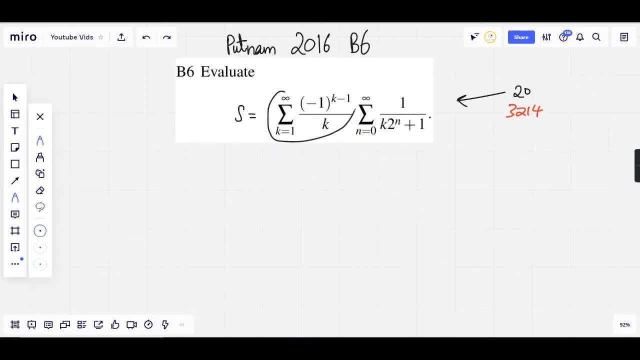 Also, one thing to note is that this summation itself is well the expression for natural log of 2. But I can't substitute that in just. I can't substitute that in just this yet, because I also have a k here. 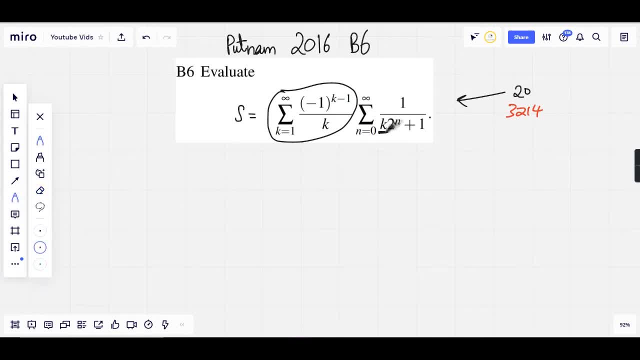 Perhaps if I were able to interchange this term into this summation somehow with the help of an integral or just anything, maybe I could use the Taylor series expansion of natural log of 1 plus x. That gives us motivation to try to represent our term here as an integral. 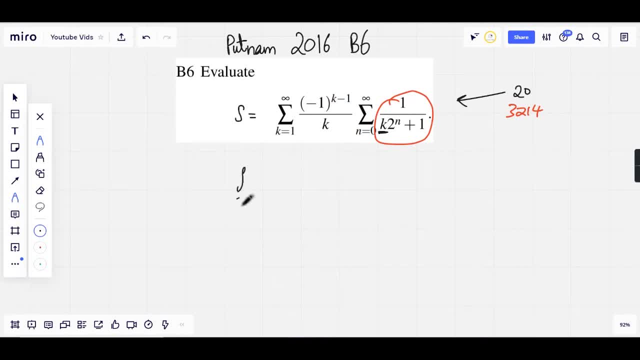 The most direct way that I can see is through integral from 0 to 1 of x to the n. dx is 1 over n plus 1.. I can replace n here with k times 2 to the n and we've got our integral representation. 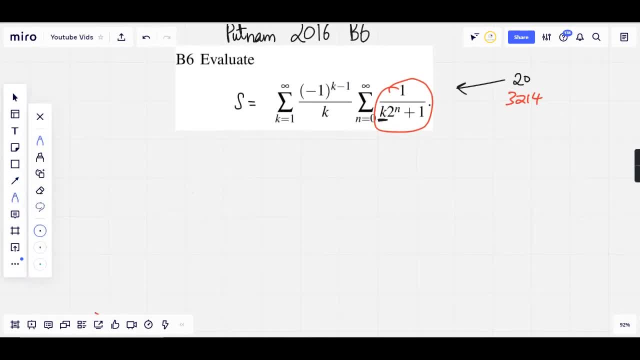 So let's rewrite the sums. then We have s equals. summation from k equals 1 to infinity minus 1 to the k minus 1 over k. Summation from n equals 0 to infinity. integral from 0 to 1 of x times k to the k times 2 to the n dx. 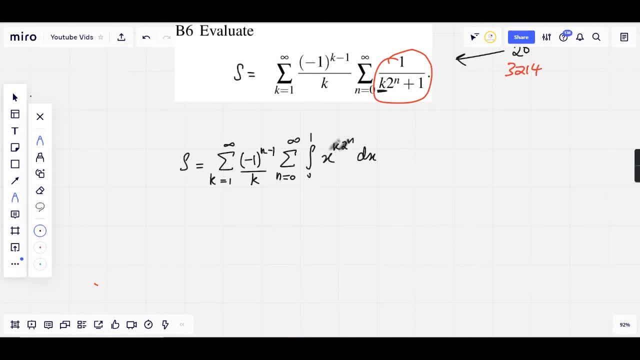 I have a power of x here now and this looks promising. I feel more inclined to using the Taylor series of natural log of 1 plus x. now Let's just swap the integrals and summations around, which we can do, because we know that the sum does indeed converge. 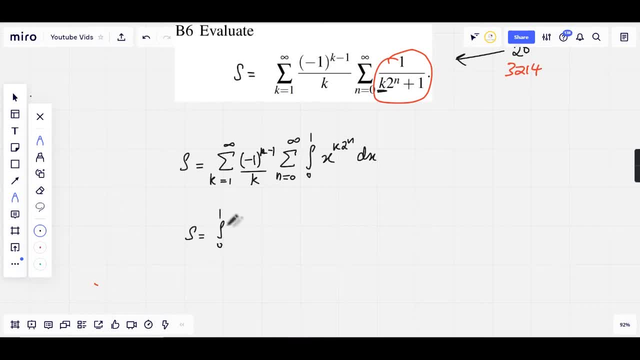 We then have s equals integral from 0 to 1, sum from n equals 0 to infinity. sum from k equals 1 to infinity, minus 1 to the k minus 1, x to the 2 to the n. all to the power of k over k dx. 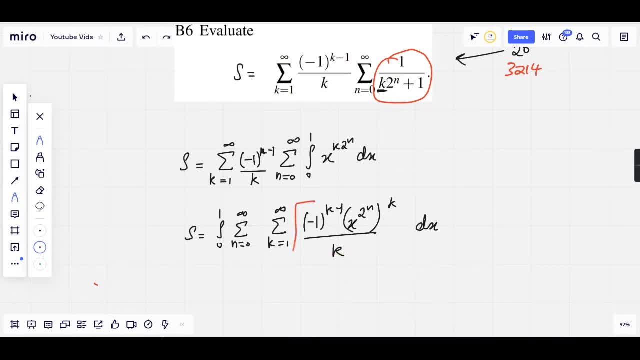 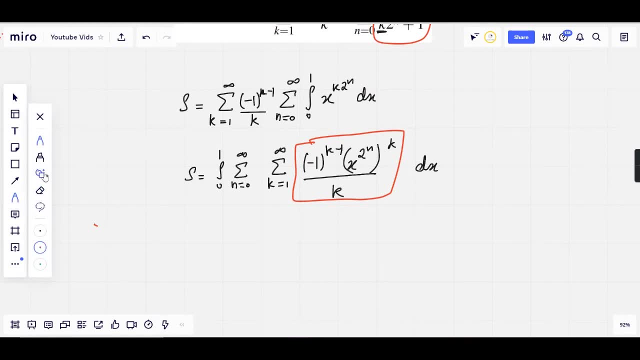 Now for those of you familiar with the Taylor series of natural log of 1 plus x. this is a direct substitution. The summation now reduces to only s equals integral from 0 to 1, sum from n equals 0 to infinity of natural log of 1 plus x to the 2 to the n. 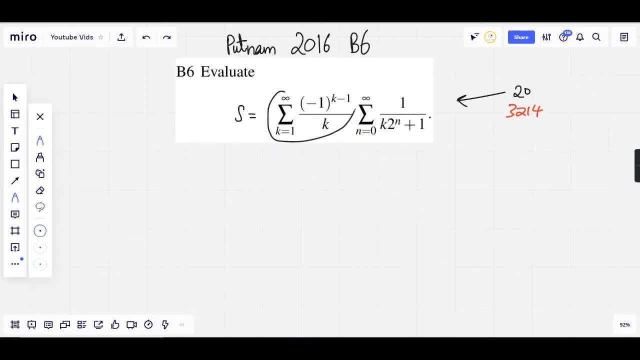 Also, one thing to note is that this summation itself is well the expression for natural log of 2. But I can't substitute that in just. I can't substitute that in just this yet, because I also have a k here. 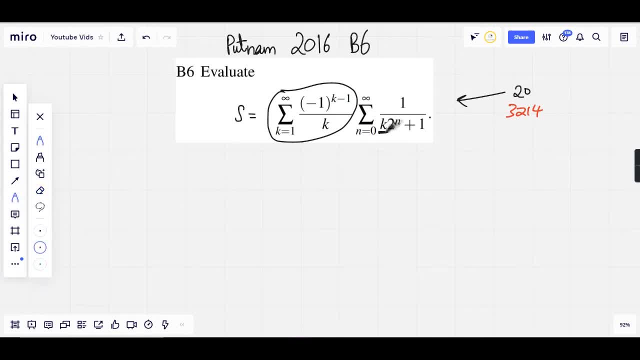 Perhaps if I were able to interchange this term into this summation somehow with the help of an integral or just anything, maybe I could use the Taylor series expansion of natural log of 1 plus x. That gives us motivation to try to represent our term here as an integral. 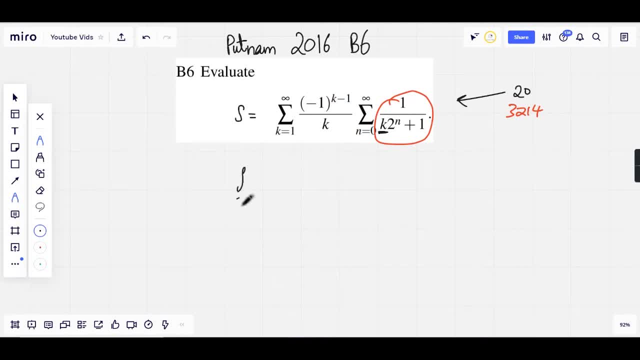 The most direct way that I can see is through integral from 0 to 1 of x to the n. dx is 1 over n plus 1.. I can replace n here with k times 2 to the n and we've got our integral representation. 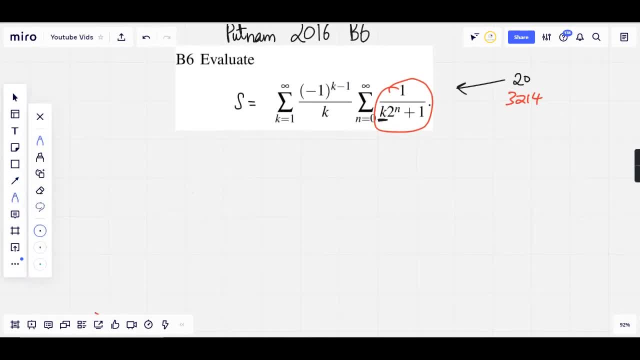 So let's rewrite the sums. then We have s equals. summation from k equals 1 to infinity minus 1 to the k minus 1 over k. Summation from n equals 0 to infinity. integral from 0 to 1 of x times k to the k times 2 to the n dx. 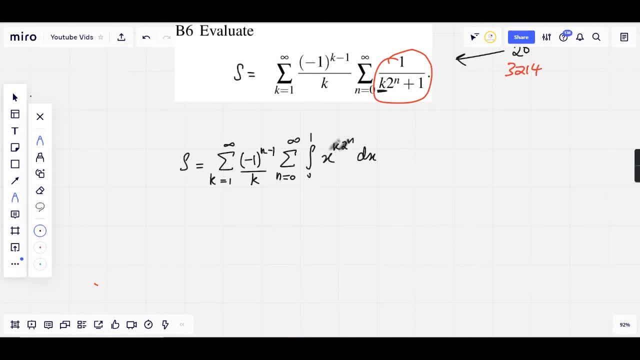 I have a power of x here now and this looks promising. I feel more inclined to using the Taylor series of natural log of 1 plus x. now Let's just swap the integrals and summations around, which we can do, because we know that the sum does indeed converge. 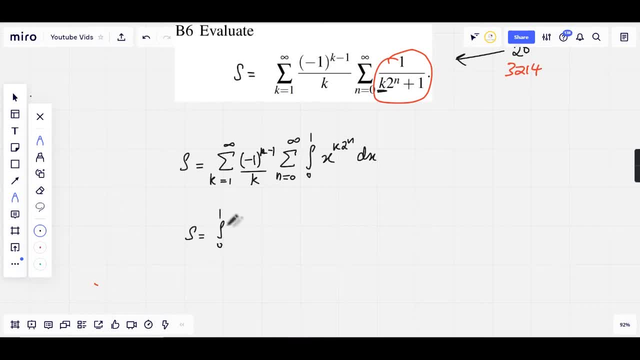 We then have s equals integral from 0 to 1, sum from n equals 0 to infinity. sum from k equals 1 to infinity, minus 1 to the k minus 1, x to the 2 to the n. all to the power of k over k dx. 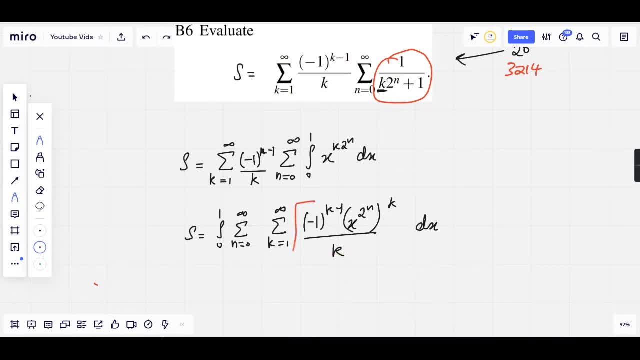 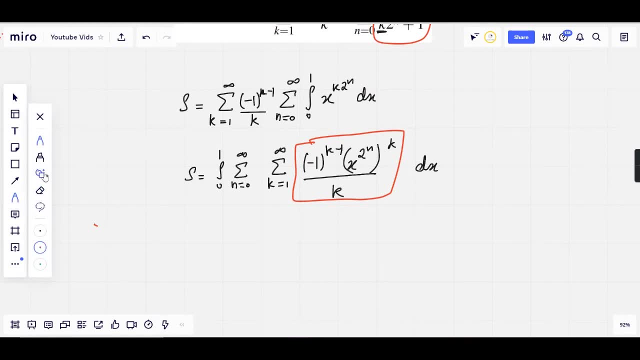 Now for those of you familiar with the Taylor series of natural log of 1 plus x. this is a direct substitution. The summation now reduces to only s equals integral from 0 to 1, sum from n equals 0 to infinity of natural log of 1 plus x to the 2 to the n. 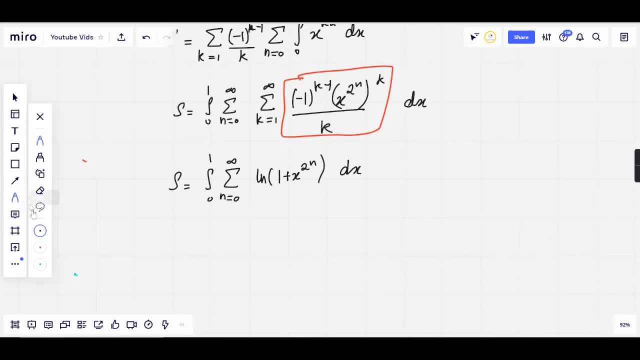 This looks a bit more manageable now, but how are we going to deal with this summation? Well, let's just write out a few terms. This would be the natural Natural log of 1 plus x, plus natural log of 1 plus x squared, and so on. 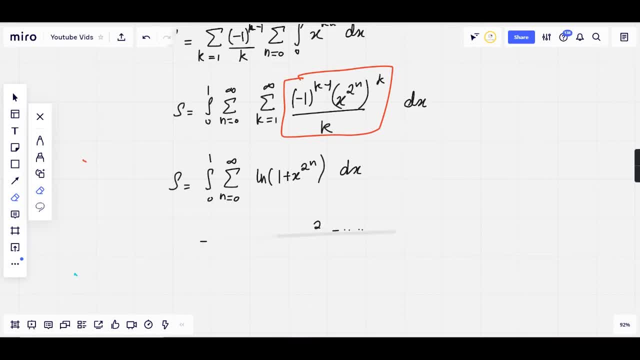 What do I know about summations and logarithms? I do know that there's this one property, namely that if I have natural log of a, b, c, that's natural log of a plus natural log of b plus natural log of c. 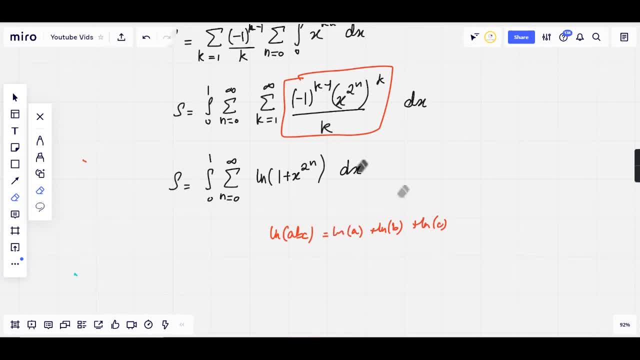 Perhaps I can do the opposite. If I have a summation, I can rewrite it as a product. Let's see where that takes us. We then have s equals integral from 0 to 1, natural log on the outside of the product, from n equals 0 to infinity, of 1 plus x to the 2 to the n dx. 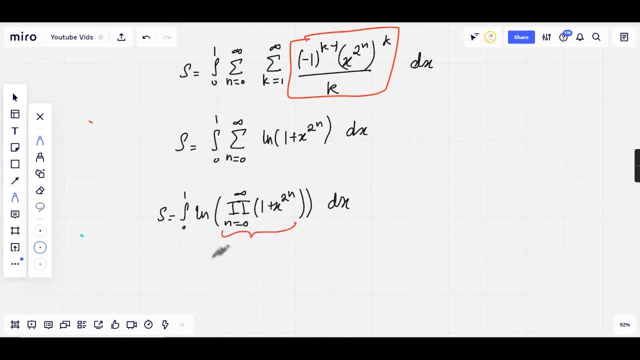 Now we're left with only doing this product, and for those of you who are familiar with Jacobi products, this is good news. For those of you who aren't, let's just write out a few terms and observe something very interesting. Well, the first term is just 1 plus x. 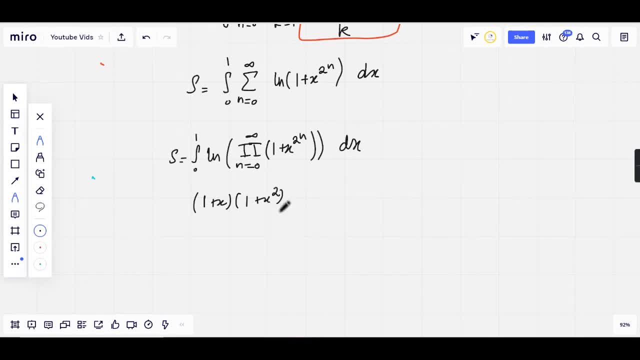 The second term multiplied would be 1 plus x squared, which gives us 1 plus x plus x squared plus x cubed. The third term, well, that would give us, if we write it out, that would be 1 plus x plus x squared, plus x cubed, plus x to the 4 plus. 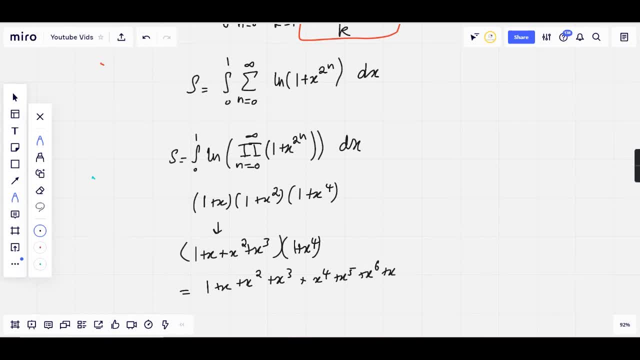 plus x to the 5, plus x to the 6, plus x to the 7, and if we put in another term, I hope you guys can see what's happening now. This 1 here it multiplies into all of these terms and gives all the powers less than 2 to the n here. and this 8 multiplies with all of these terms and gives all the power up to the next 2 to the n plus 1.. 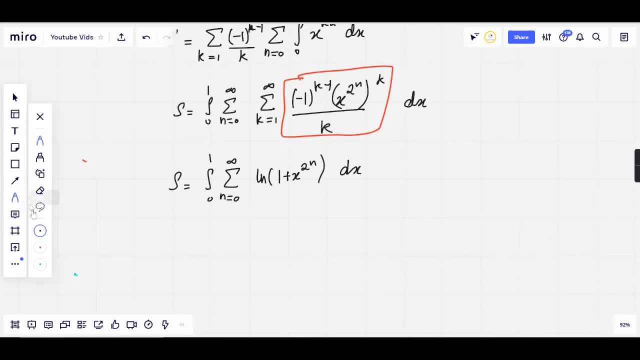 This looks a bit more manageable now, but how are we going to deal with this summation? Well, let's just write out a few terms. This would be the natural Natural log of 1 plus x, plus natural log of 1 plus x squared, and so on. 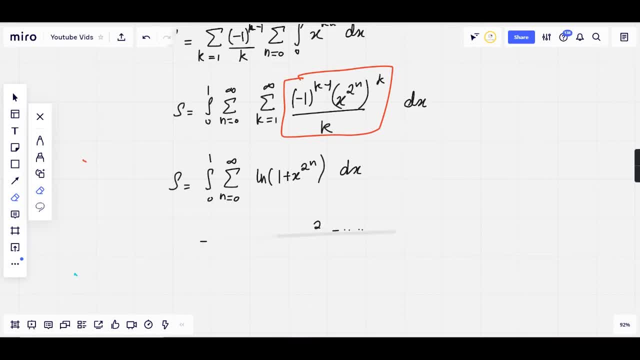 What do I know about summations and logarithms? I do know that there's this one property, namely that if I have natural log of a, b, c, that's natural log of a plus natural log of b plus natural log of c. 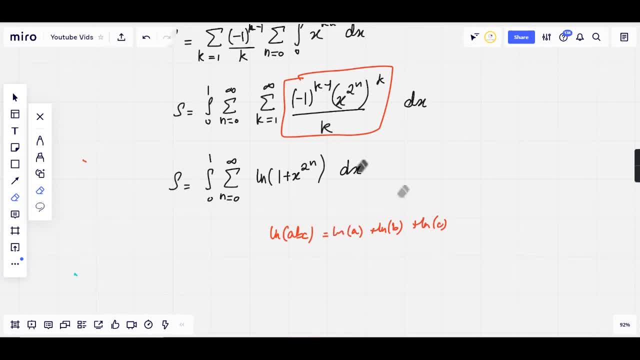 Perhaps I can do the opposite. If I have a summation, I can rewrite it as a product. Let's see where that takes us. We then have s equals integral from 0 to 1, natural log on the outside of the product, from n equals 0 to infinity, of 1 plus x to the 2 to the n dx. 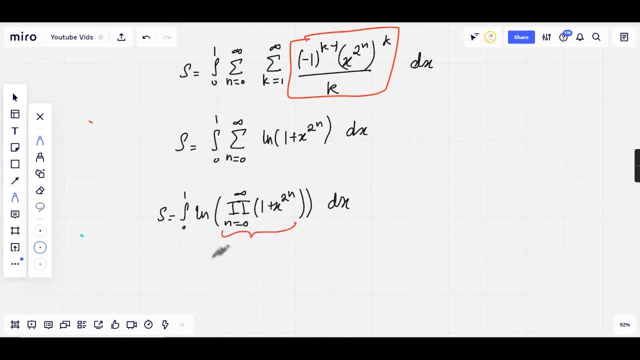 Now we're left with only doing this product, and for those of you who are familiar with Jacobi products, this is good news. For those of you who aren't, let's just write out a few terms and observe something very interesting. Well, the first term is just 1 plus x. 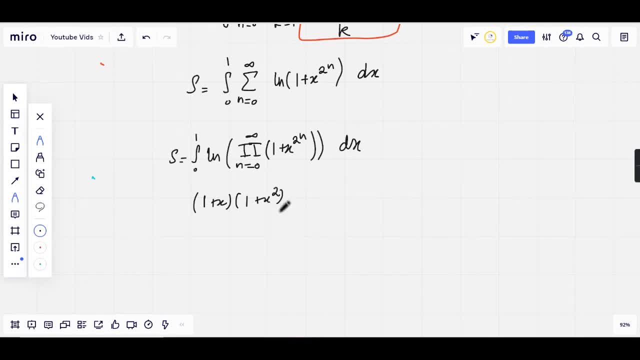 The second term multiplied would be 1 plus x squared, which gives us 1 plus x plus x squared plus x cubed. The third term, well, that would give us, if we write it out, that would be 1 plus x plus x squared, plus x cubed, plus x to the 4 plus. 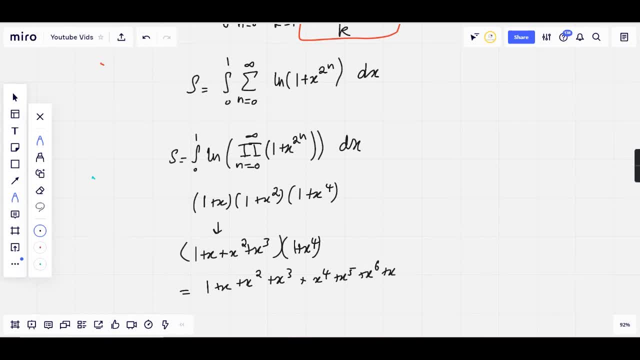 plus x to the 5, plus x to the 6, plus x to the 7, and if we put in another term, I hope you guys can see what's happening now. This 1 here it multiplies into all of these terms and gives all the powers less than 2 to the n here. and this 8 multiplies with all of these terms and gives all the power up to the next 2 to the n plus 1.. 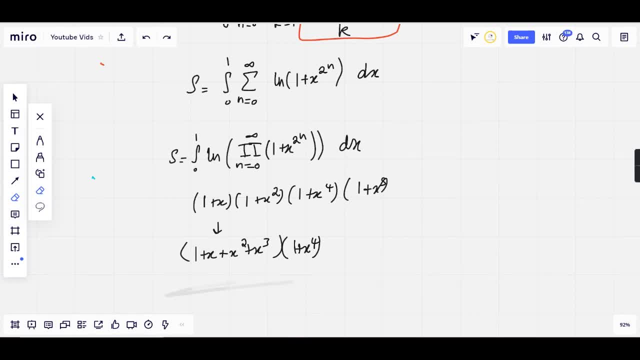 So this gives us all the powers up to 2 to the n, and this can be done by induction, As we have an infinite sum. well, it's going to give us all the powers of 2, and, well, actually, all the powers of x. 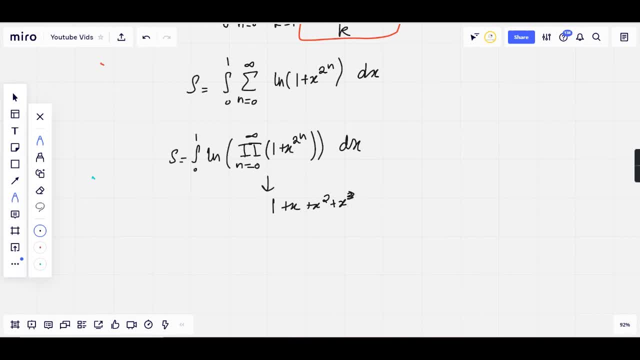 So we see that this summation, or sorry, this product, reduces to just this infinite series. We know that our domain is 0 to 1, and the value of x less than 1, this geometric series converges to 1 over 1 minus x. 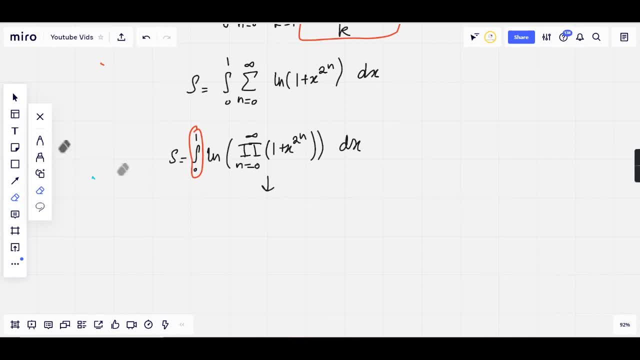 I can then rewrite this problem and it becomes a very classic integral. then S equals the integral from 0 to 1 of natural log of 1 over 1 minus x. Well, from the properties of natural logarithm, I can rewrite this as: 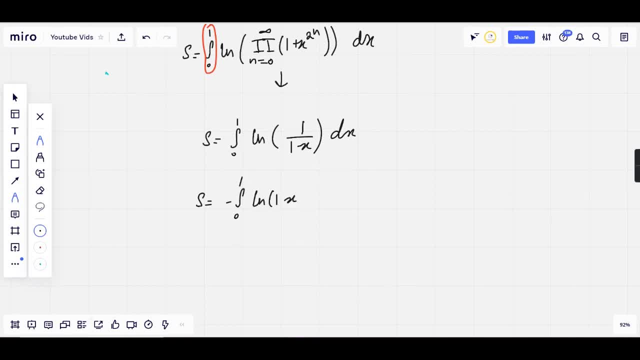 the negative of 0 to 1 of natural log of 1 minus x. This is a trivial integral that you can do by substituting: u equals 1 minus x. Let's do that. The limits then would change. You have dx over du equals negative 1.. 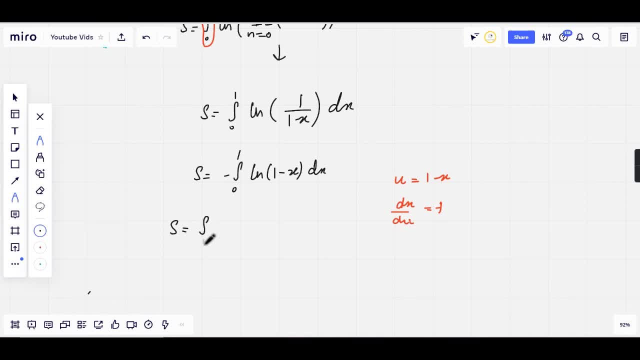 So you'd have s equals integral from 1 to 0 of natural log of u du, which would then be u natural log of u minus u from 1 to 0.. I know that the limit, as u goes to 0 of natural log of u to the u is 0. 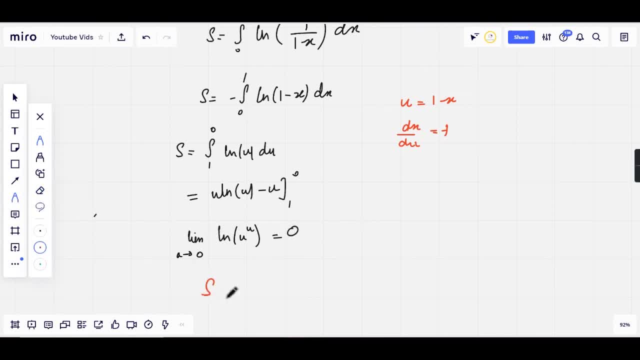 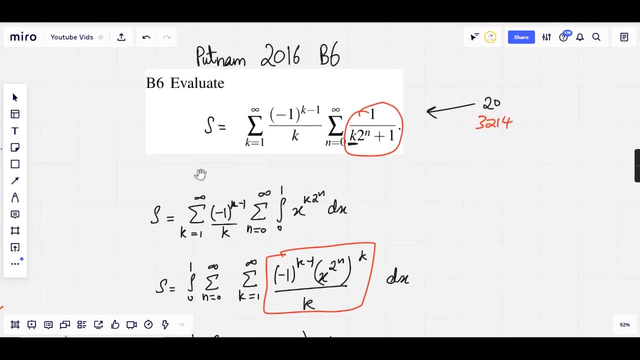 So the answer that we're left with is s equals minus minus 1,, which is 1.. The answer to our daunting summation is a whopping 1.. That was B6 of Putnam 26. A seemingly challenging problem. That's the end of the video. 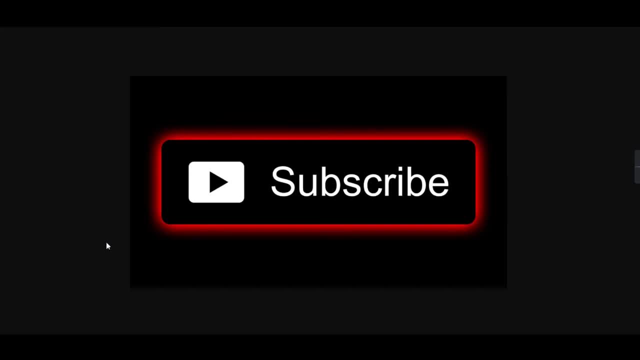 I hope you guys did enjoy the video. If you did, please do leave a like and a comment letting me know what you liked most. If you didn't, please do leave a comment letting me know how to improve. I'm always open to hearing your suggestions. 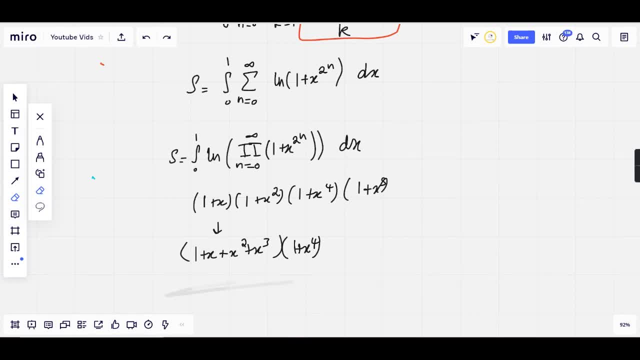 So this gives us all the powers up to 2 to the n, and this can be done by induction, As we have an infinite sum. well, it's going to give us all the powers of 2, and, well, actually, all the powers of x. 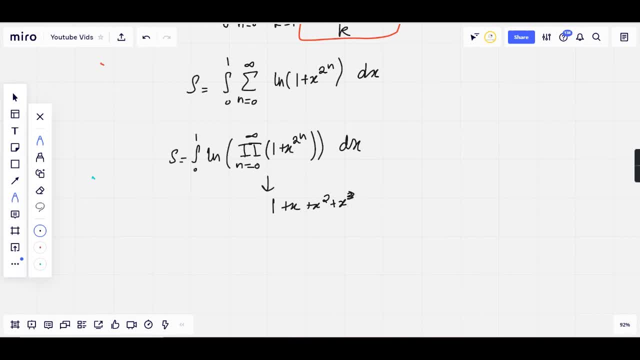 So we see that this summation, or sorry, this product, reduces to just this infinite series. We know that our domain is 0 to 1, and the value of x less than 1, this geometric series converges to 1 over 1 minus x. 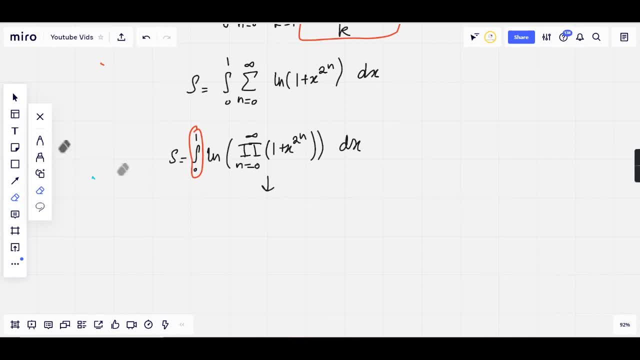 I can then rewrite this problem and it becomes a very classic integral. then S equals the integral from 0 to 1 of natural log of 1 over 1 minus x. Well, from the properties of natural logarithm, I can rewrite this as: 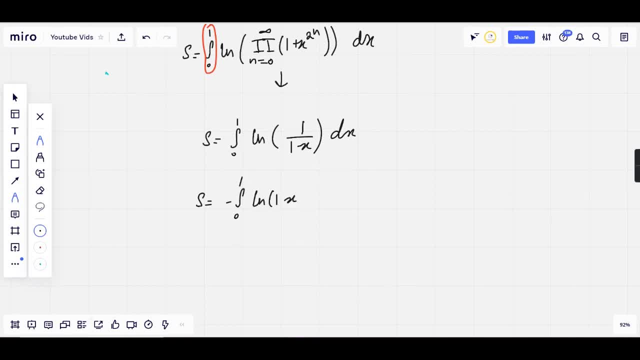 the negative of 0 to 1 of natural log of 1 minus x. This is a trivial integral that you can do by substituting: u equals 1 minus x. Let's do that. The limits then would change. You have dx over du equals negative 1.. 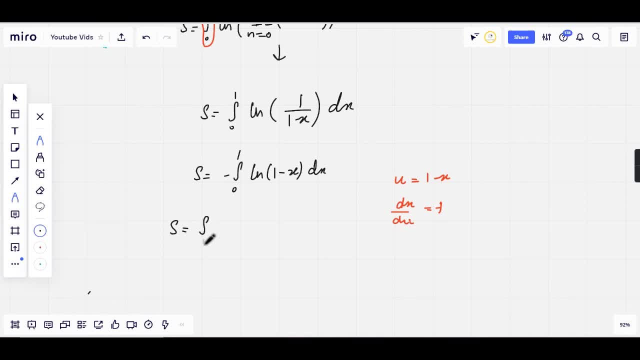 So you'd have s equals integral from 1 to 0 of natural log of u du, which would then be u natural log of u minus u from 1 to 0.. I know that the limit, as u goes to 0 of natural log of u to the u is 0. 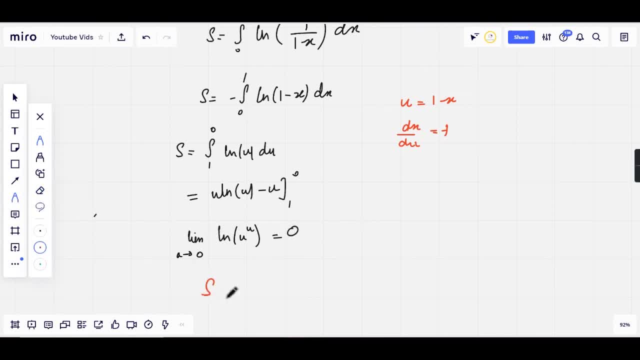 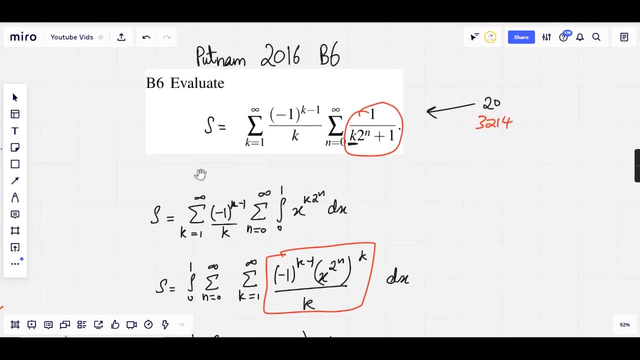 So the answer that we're left with is s equals minus minus 1,, which is 1.. The answer to our daunting summation is a whopping 1.. That was B6 of Putnam 26. A seemingly challenging problem. That's the end of the video. 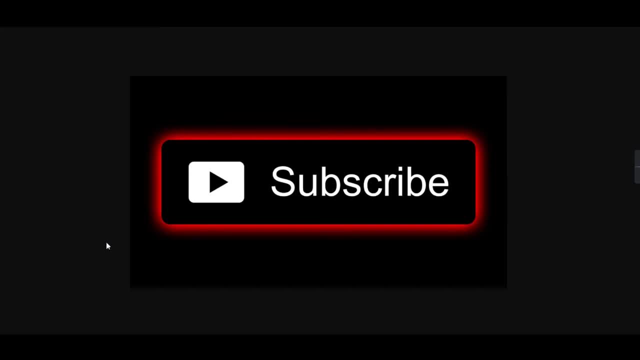 I hope you guys did enjoy the video. If you did, please do leave a like and a comment letting me know what you liked most. If you didn't, please do leave a comment letting me know how to improve. I'm always open to hearing your suggestions.